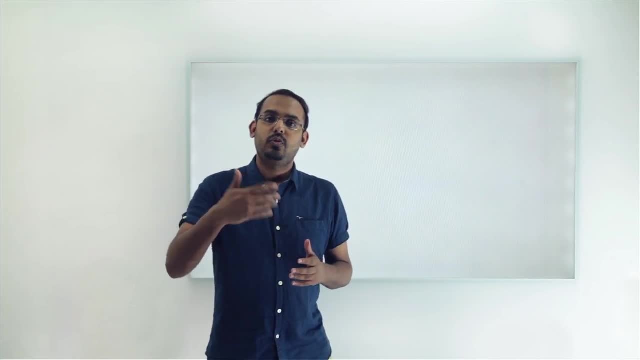 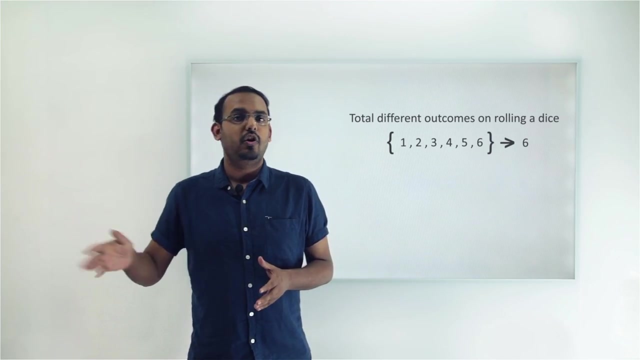 So let's analyze this step by step. So when you roll the dice, there are six different possibilities of you getting a result. So you can get any one of the numbers from one to six. Now you know that you will win only if you roll the numbers four, five or six. 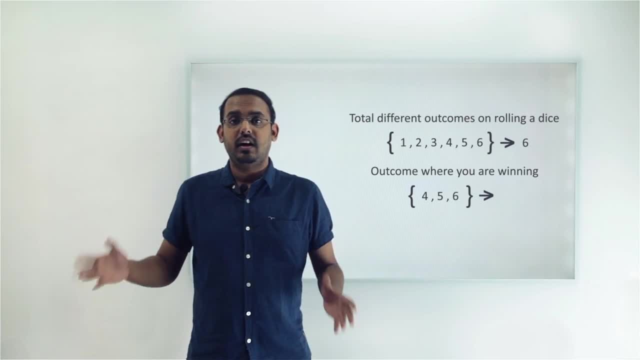 So if you look at this, out of the six different outcomes that you can get when you roll a dice, there are three outcomes that lead to the result of you winning the game. So if you think about it logically, you can say that there are three out of six different ways in which you can win the game. 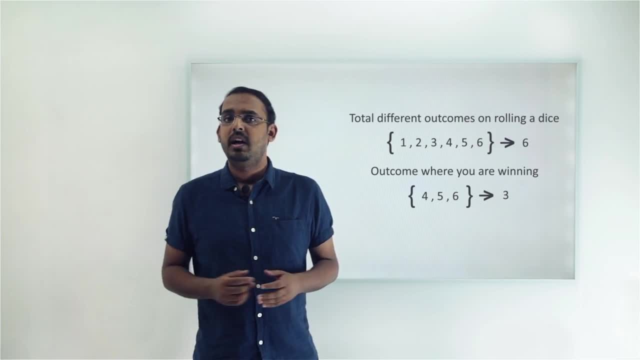 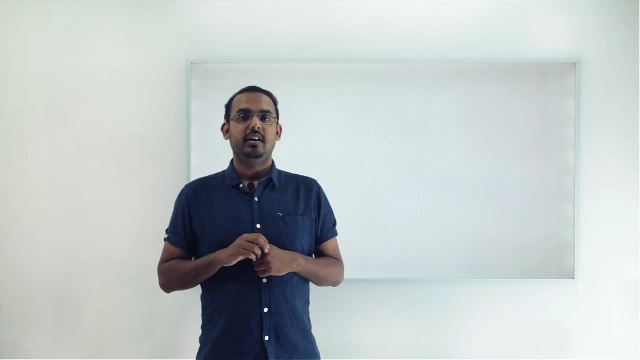 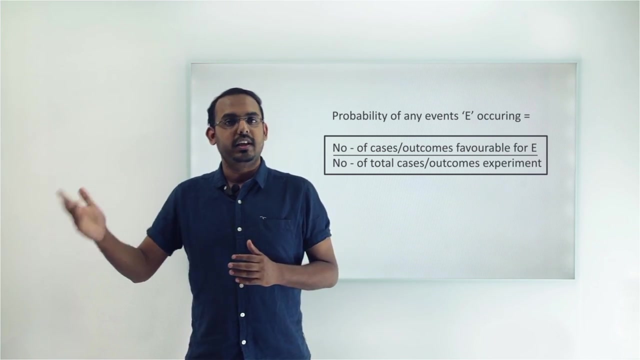 So the chances of you winning the game are three out of six. So this is exactly what the theory of probability also tells us. So, according to the theory of probability, the probability of an event E- occurring is given by the ratio of the value of the total number of events favorable to E and 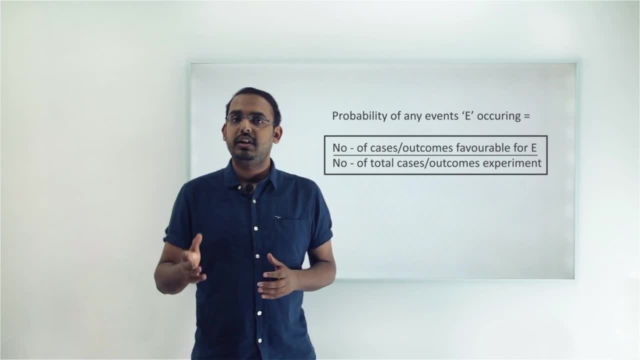 the value of the total number of events associated with the experiment. So if you look at that formula now and if you try to use it in our scenario, what you can see is that the number of favorable events for you winning the game are three, as we saw earlier. 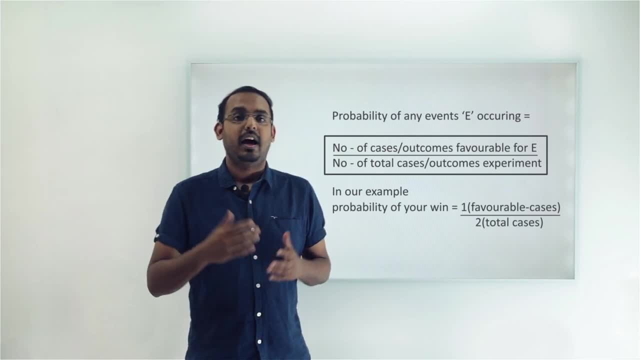 And the total number of events when you roll a dice are six. 6 because you can get any of the numbers from 1 to 6.. So if you use this definition of probability, you will get your chances of winning as 3 by 6, which is the same as we figured out earlier. 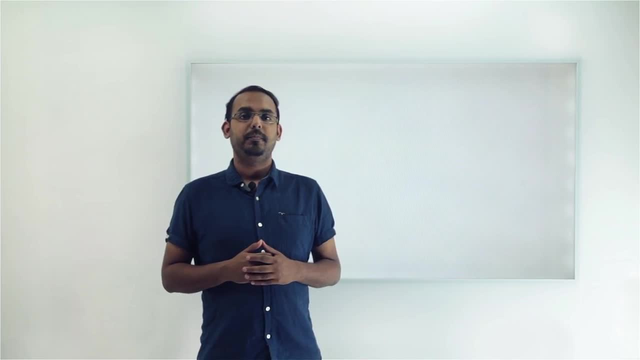 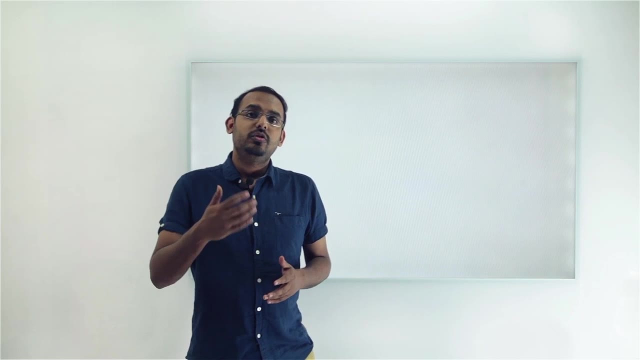 So this is the concept of theoretical probability. Now let's take another example to understand the concept of theoretical probability. So suppose you and your friend's team, your team and your friend's team, are playing a cricket match and you are walking out on the pitch for the coin toss. 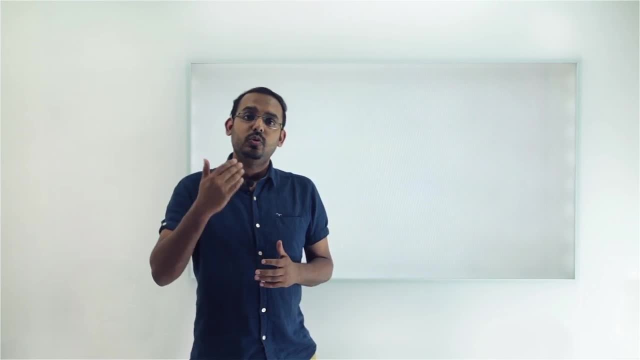 Now your friend calls the value tails. So you know that you can win the coin toss if you get a heads right Now, what is the probability that you will win the coin toss? So to calculate this, let us analyze this whole scenario again. 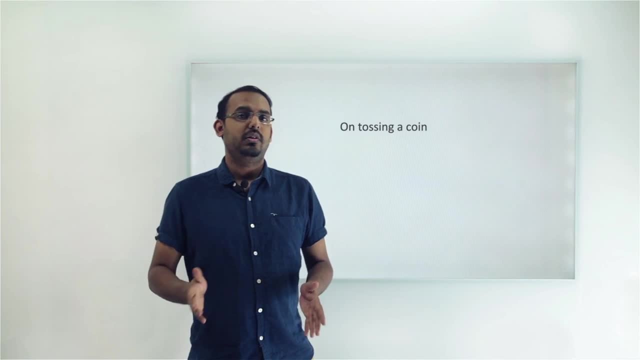 So when we toss a coin, we have two different possible outcomes. We can get either heads or tails. Now, since your friend has already called for getting tails, you know that you will win the coin toss when you get a heads. So the number of cases in which you can win are 1.. 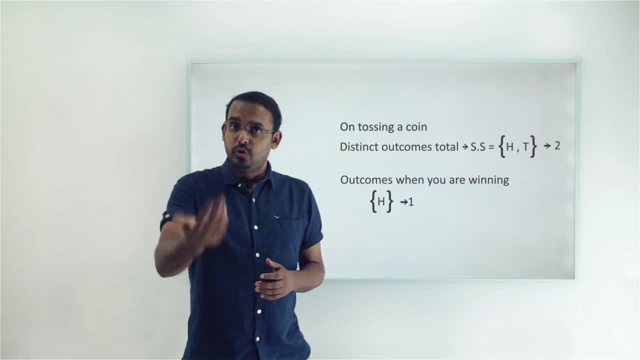 So we can also say that the number of favorable cases to you winning the coin toss is 1. And the number of total cases or the number of total outcomes that are possible when you toss a coin are 2.. So if we use the same definition of theoretical probability again here, 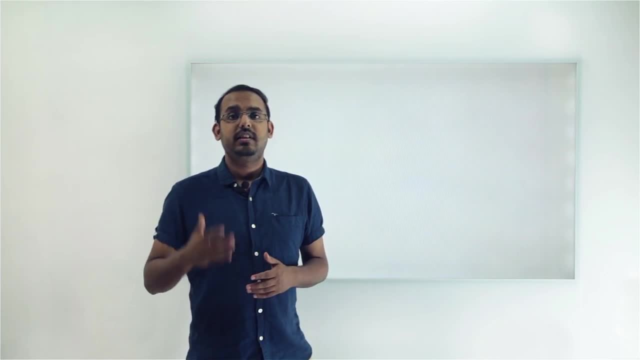 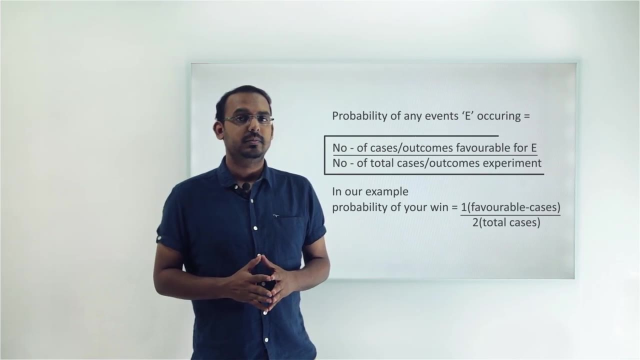 We can see that the probability says that the chances of you winning are 1 by 2. So there is a 50% chance that you will win the coin toss, But we know that this doesn't happen in our real life, right. 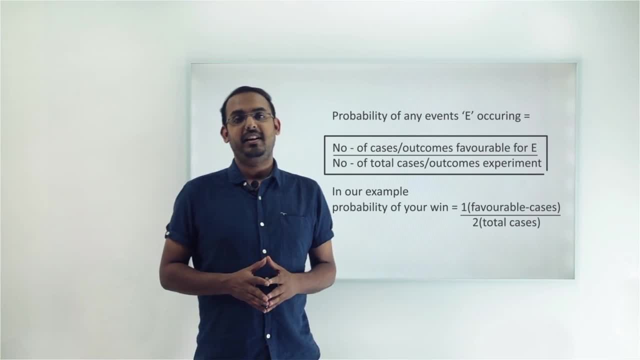 So I, for one, remember losing countless coin tosses in my life. So why does this happen when we know that our chances of winning the coin toss are clearly 1 out of 2?? So now to understand about experimental logic, Let's start with the first one. 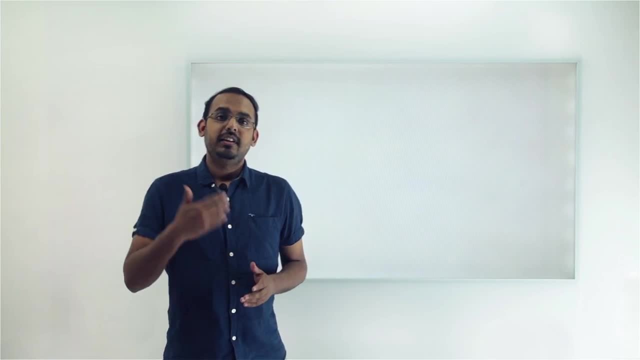 The theoretical probability. Let's perform a small experiment. So in this experiment, I have a coin with me and I'll toss this coin 10 times And we'll catch it and see what the result is. Now, by the definition of theoretical probability, I should be getting 5 times heads and 5 times. 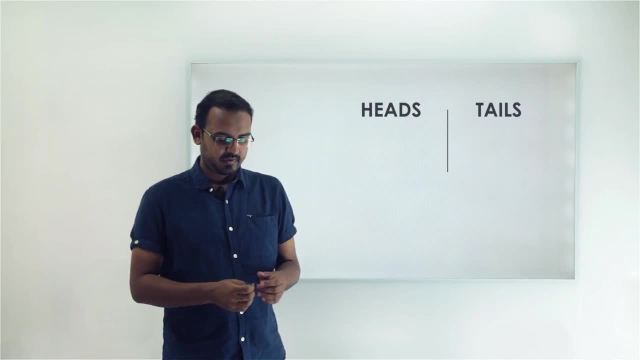 tails. Let's see if that actually happens. So the first time I toss the coin I get the value tails. So I get 1 tails Heads this time. So 1 heads Tails, So tails becomes 2. Tails again. 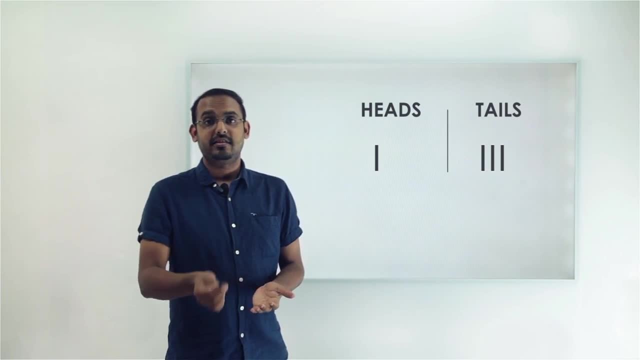 So tails becomes 3.. Heads this time. So heads becomes 2.. So I've tossed the coin 5 times and 3 times I've got tails and 2 times I've got heads. Now let's continue this experiment: Heads this time. 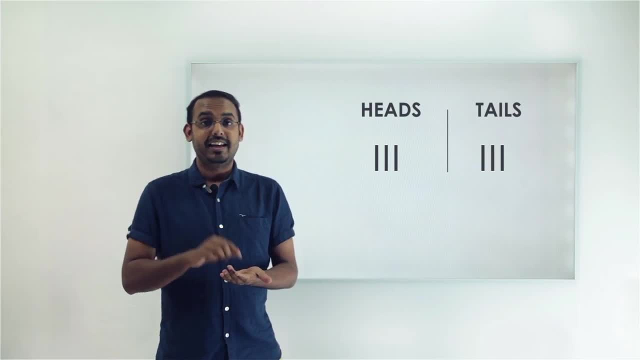 So 3 times tails, 3 times heads, Tails this time. So 4 times tails, 3 times heads, Again tails. 5 times tails, 3 times heads, Tails again. So currently it stands at 6 times tails and 3 times heads. 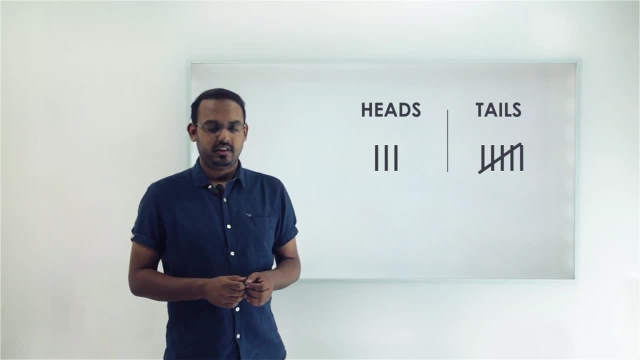 Tails again. So I've completed this experiment 10 times and 7 out of those times I've got the value tails and 3 out of those times I've got the value heads. So does this mean that the definition of theoretical probability gives us the wrong result? 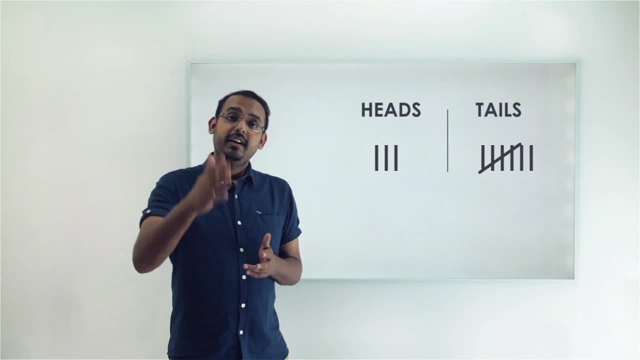 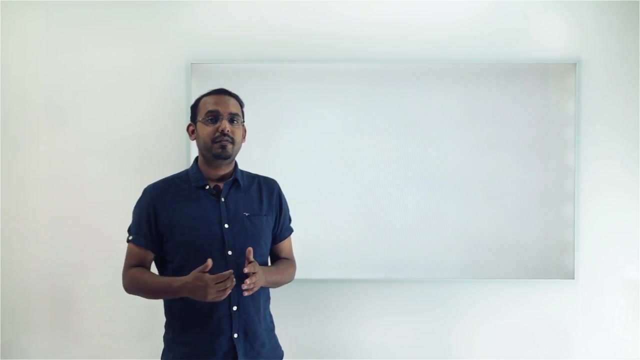 No, Well, theoretical probability gives us an idea about what to expect when we perform the experiment. In experimental probability approach, we actually perform the experiment first and try to find the probability by recording all the findings about the experimental outcomes that we have. So now these two values might vary a little. 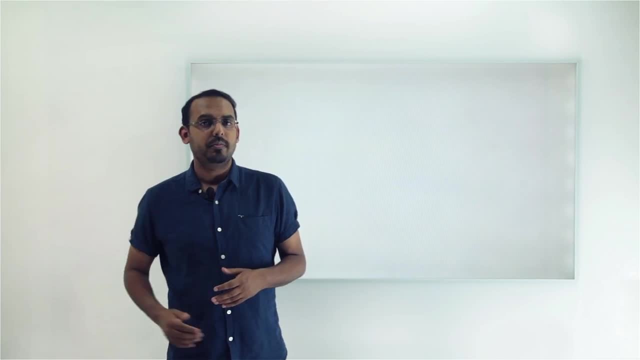 But as we keep on increasing the number of times that we perform the experiment, what we'll observe is That these two values start to move towards each other and coincide at the theoretical probability point. So why don't we always calculate experimental probability? Because we don't always have the leisure to invest that kind of time and do the experiment. 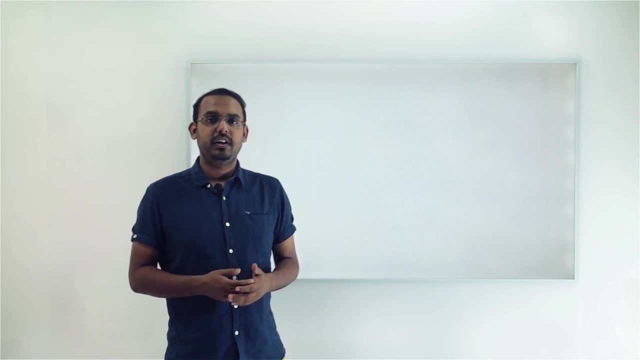 so many different times. So, for example, we perform the experiment of tossing a coin 10 times here, But I cannot go on and perform that same experiment a thousand times. I mean I can, But then we wouldn't be shooting this video for you guys, right? 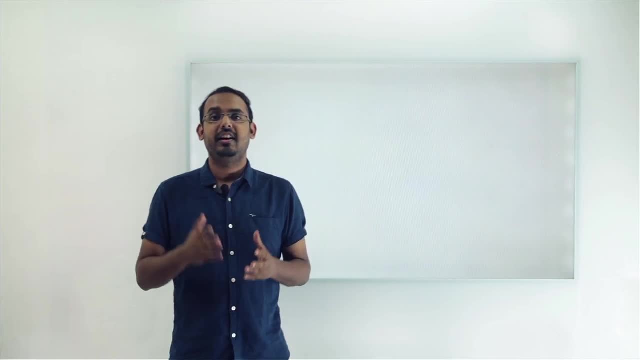 Because I'll have to invest a lot of time in tossing the coin 10,000 times or thousand times and recording all the findings. So I generally take the theoretical approach. Now, if we talk about the experimental probability and how we actually calculate it, we can see: 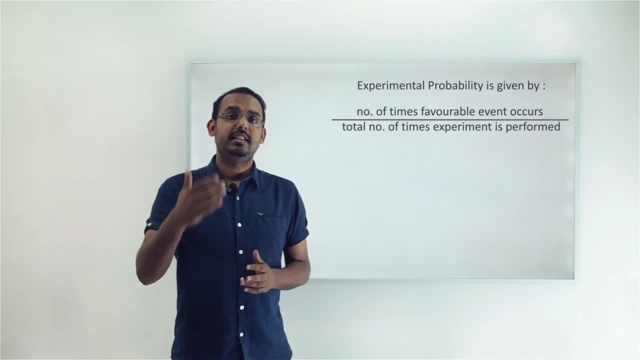 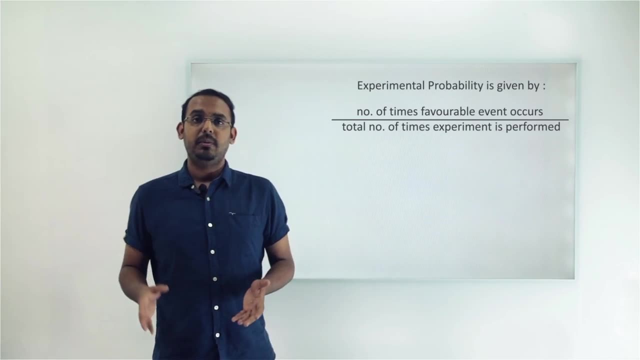 that the experimental probability, by definition, is given by the ratio between the values of the number of times- The outcome of the experiment that we performed Was favorable to our case- and the value of the number of times that we performed the experiment. So, if we take the example that we took here, we had performed the experiment of tossing. 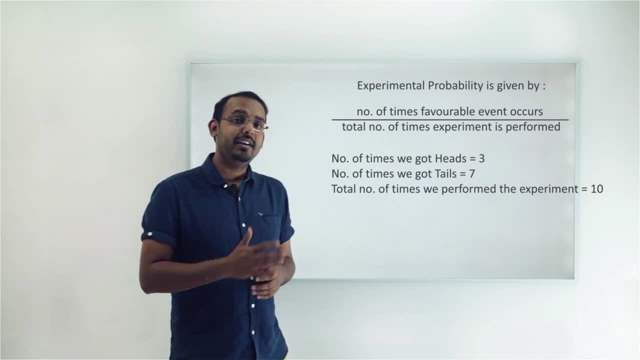 the coin 10 times and out of those 10 times, seven times, I got the value tails. So the probability, or the experimental probability, of me getting a tails when I toss the coin 10 times is going to be seven, which is the number of favorable events here. 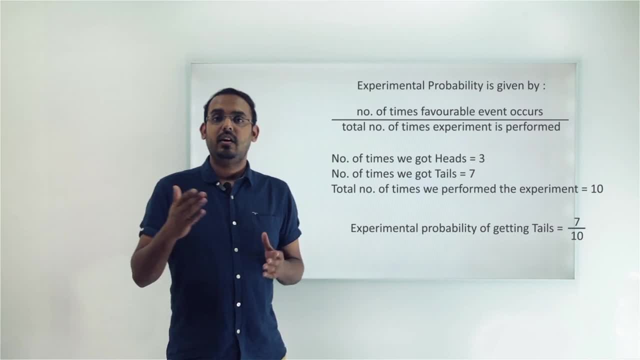 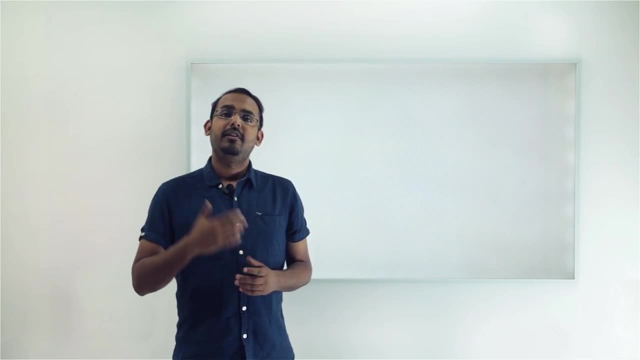 Out Out of 10, so seven by 10.. So that is how we calculate the experimental probability. Since we cannot always perform the experiment a large number of times, we'll be dealing with theoretical approach to probability. more So, whenever I use the term probability now onwards, we can inherently assume that I'm 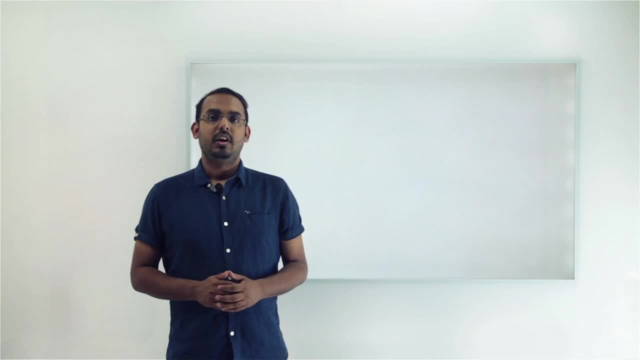 talking about the theoretical approach to probability. So this is the overall concept and how we calculate probability and what it actually means. Now Let's look at some interesting properties that probability shows. So the first important thing that we should be aware of, or we should understand, is that 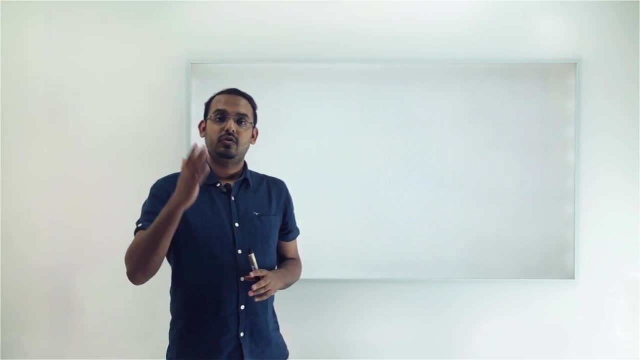 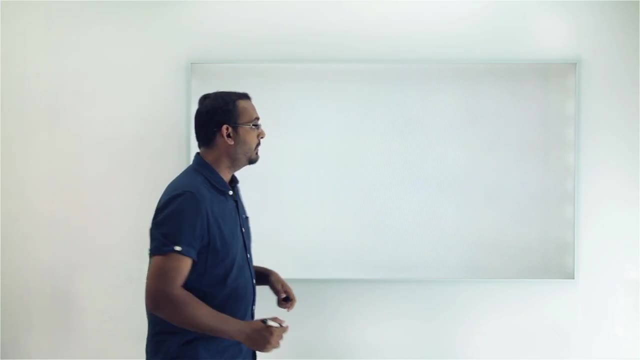 the value of probability. when we calculate it, it is always going to lie between zero and one, zero and one, both included. So we can say that probability of any event E is always going to be less than equal to one and it's always going to be greater than equal to zero. 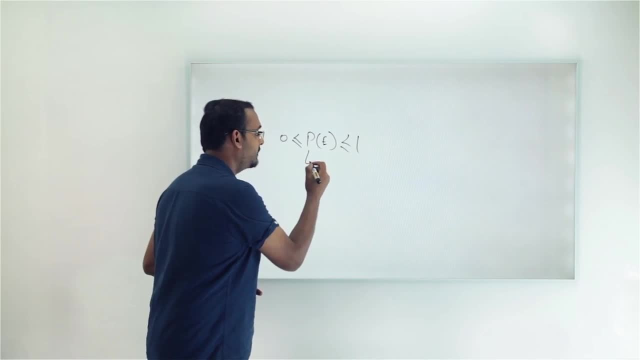 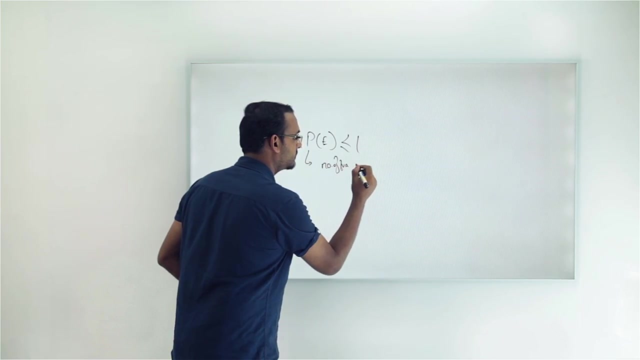 Now, How can we say that? So we know that, by definition, the value of probability of any event E occurring is given by the ratio of two values. So it's given by the ratio of number of favorable cases upon the number of total cases. 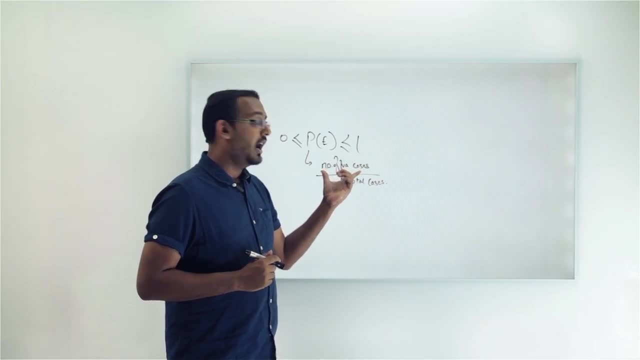 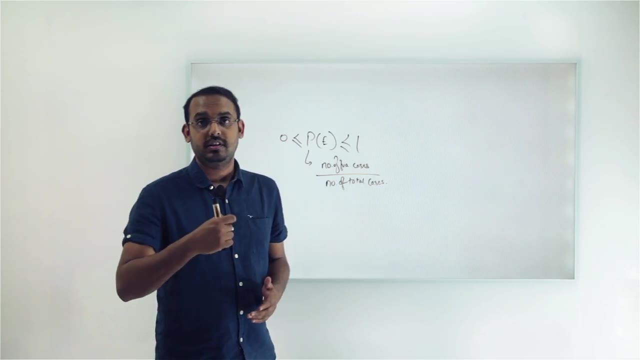 So now We know that The number of favorable cases are always going to be a subset of the total cases. So if I perform the experiment of tossing the coin and I'm trying to figure out the probability of getting a heads, So getting heads will always be one of the outcomes of performing the experiment of tossing. 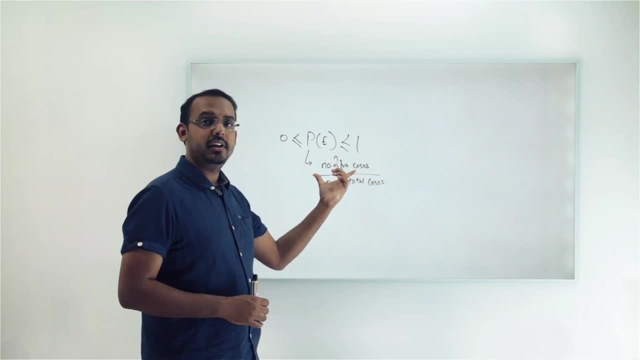 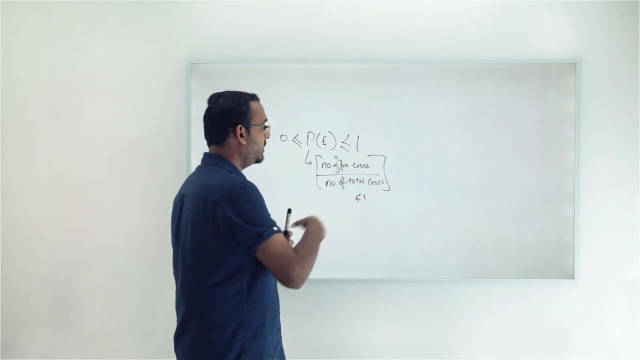 the coin. So the number of favorable cases is always going to be less than or equal to the number of total cases. So this value, this ratio, is always going to be less than or equal to one, because this value is always less than or equal to this value. 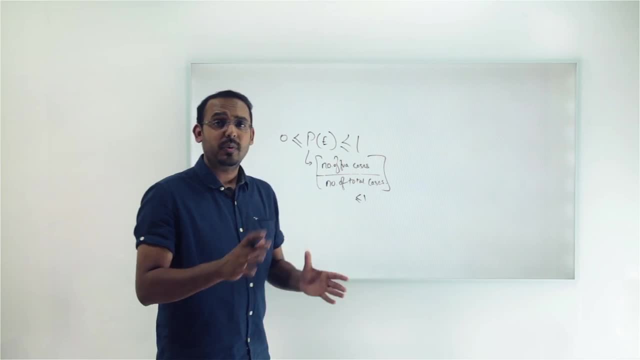 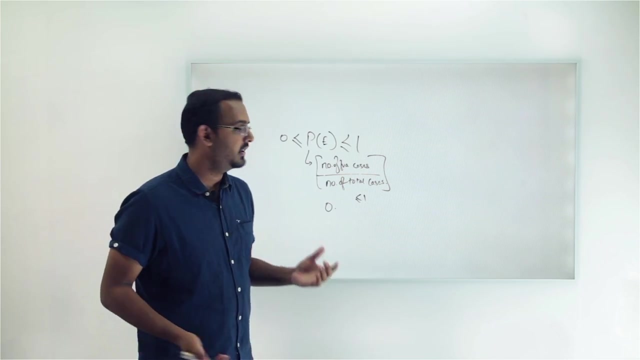 Now, if you look at the number of favorable cases, the least value this particular thing can take is going to be zero, right? Because when I'm counting something, when I'm counting the number of favorable cases for an experiment, for an event of an experiment, I cannot get a negative value for that. 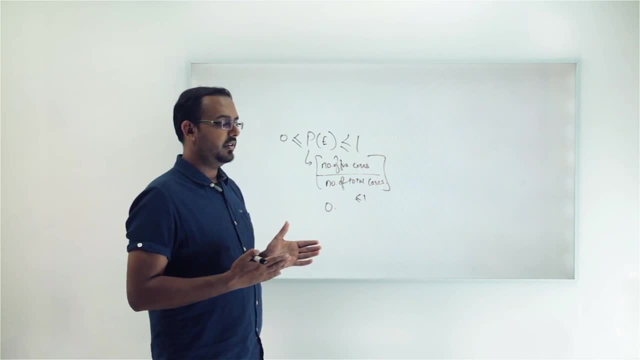 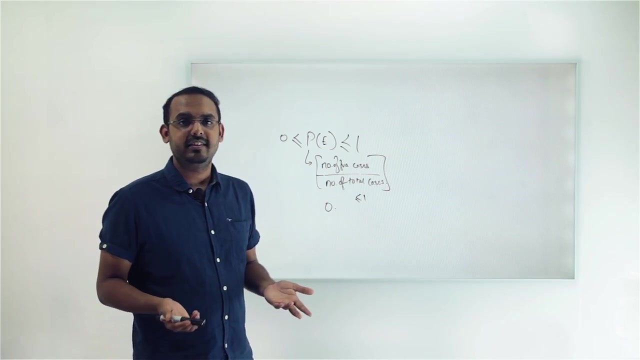 The least Value I can take is zero, right? So if we take an example of that case, suppose if we roll a dice and I say that we need to calculate the probability of getting a number which is greater than seven, So now all the numbers in the outcome, one to six, are all less than seven. 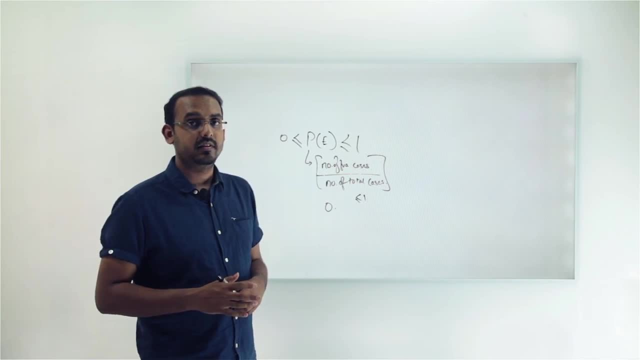 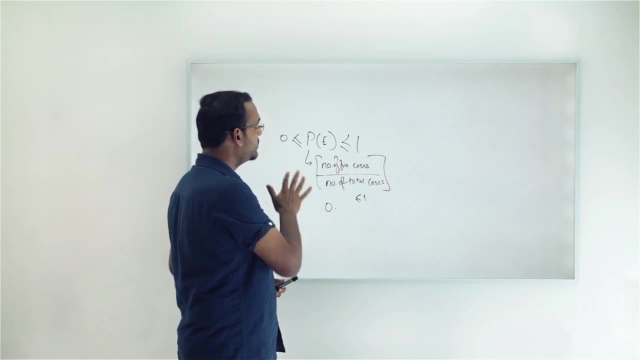 So there is no favorable case where I get a number greater than seven. So in such a case, the number of favorable cases is going to be zero. So this ratio is always going to be greater than zero, Greater than Or equal to zero. 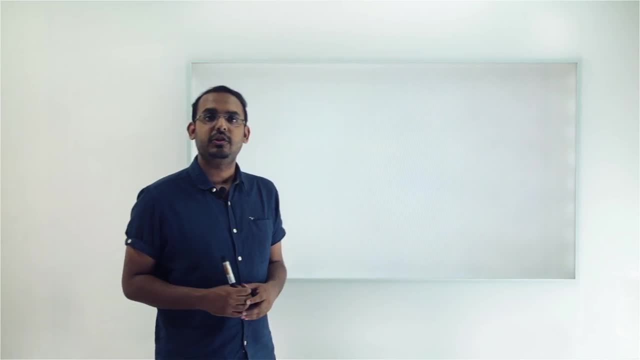 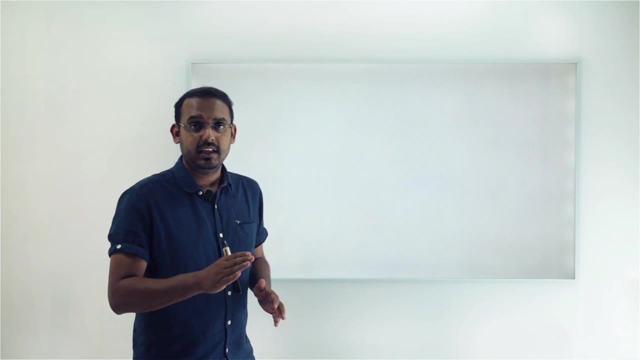 So now let's talk about the second interesting property that probability shows that we should be aware of. So this property says that the probability of any event E occurring when you're performing some experiment, plus the probability of this particular event E not happening, is always going to be the value one. 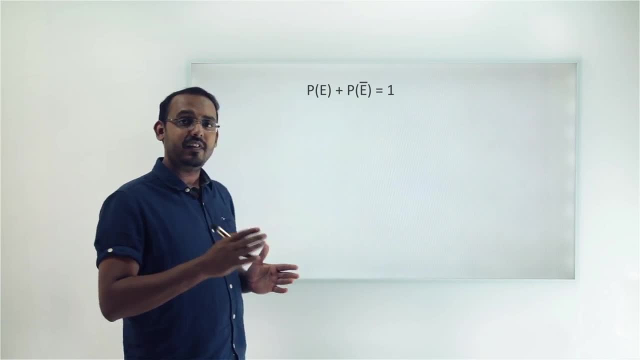 So, no matter what is the experiment that we are doing, if we have any event E in that experiment and we calculate the probability of that event happening and we calculate the probability of that event not happening, the summation of these two values is always going. 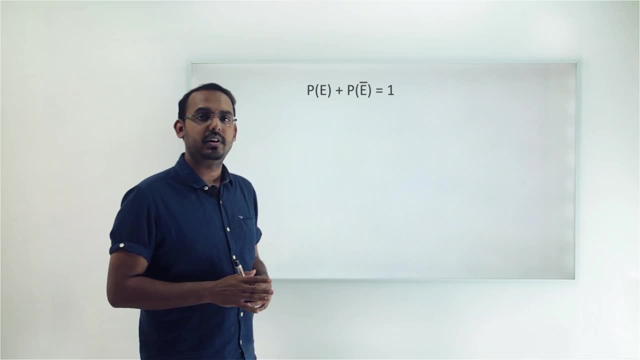 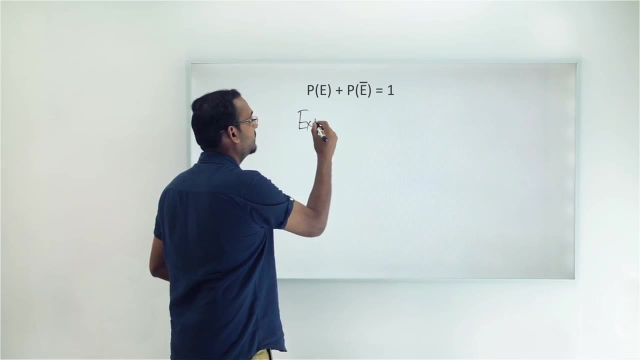 to be the number one. So now let's try to prove this property by using a very generic experiment. So let's say that the experiment that we are performing is the experiment A. Now, in this experiment, when we perform this experiment, Let's take that we get a total of t outcomes. 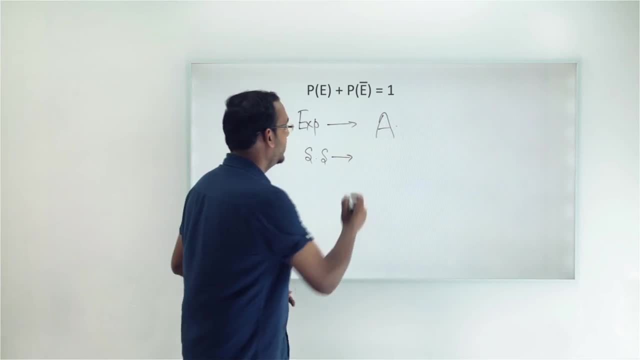 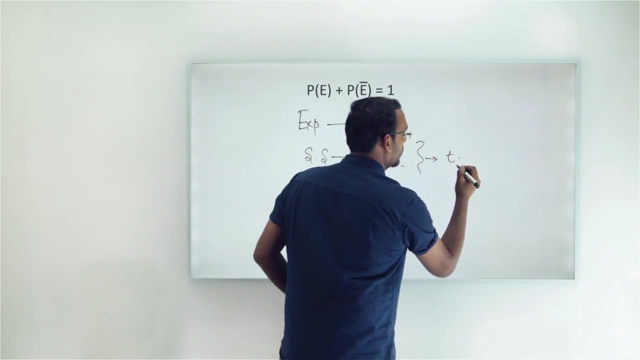 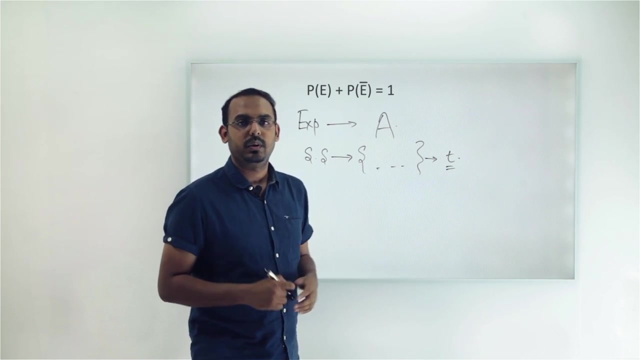 So the sample space that we get for this experiment is a set of some values, and this sample space contains a total of small t outcomes. So when we perform the experiment A, there are t distinct outcomes that we can get. Now let's take an event E. 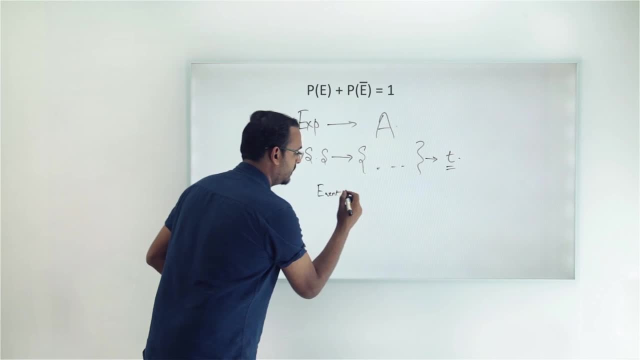 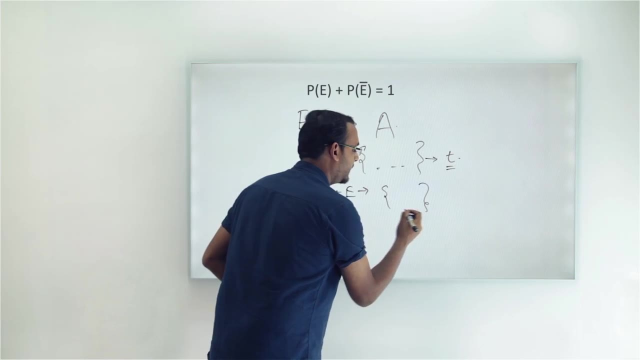 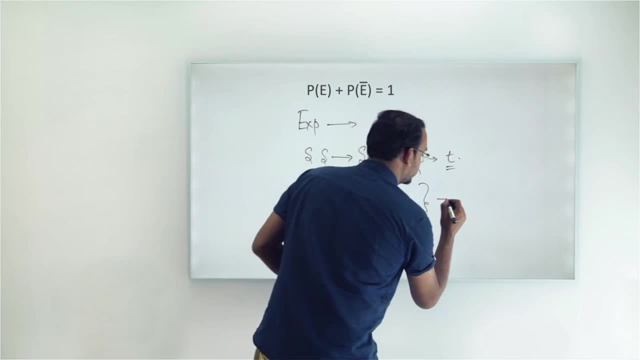 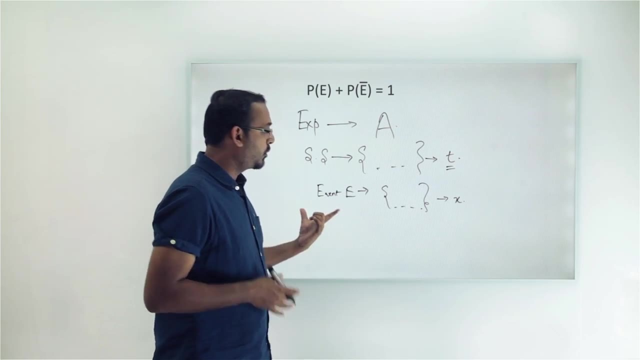 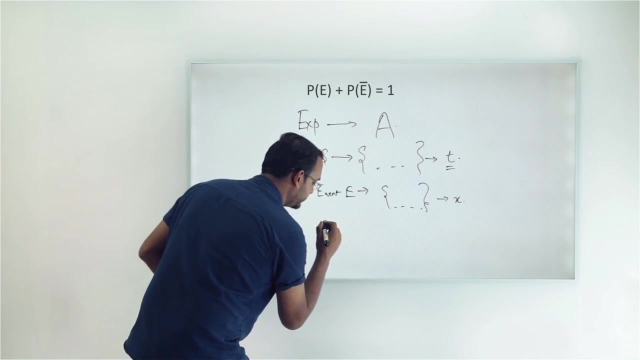 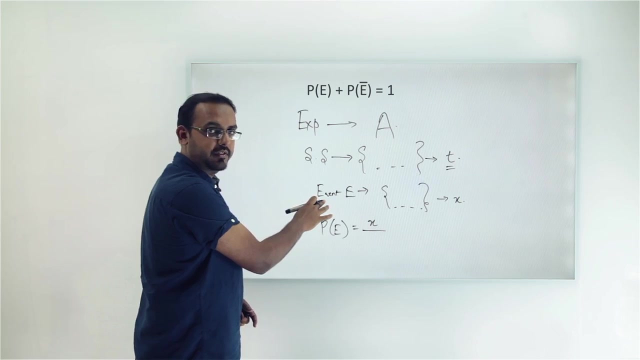 the criteria put forth by the event E is x. So if we look at this scenario now, the probability, if we try and calculate the probability of the event E happening, we can get that value as x, x, Which is the number of favourable cases for the event E happening upon T. 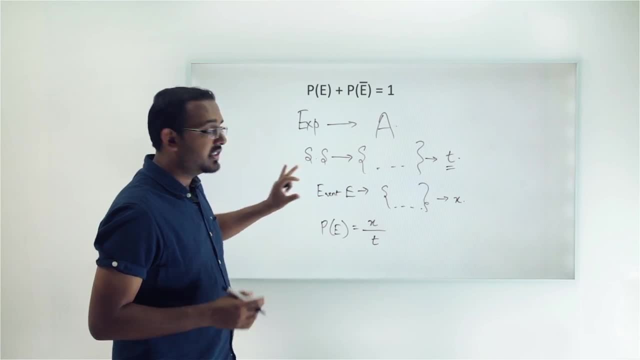 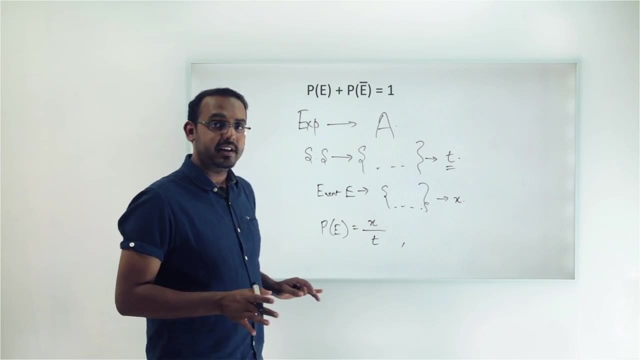 Which is the number of favourable cases, which is the number of total cases which are present in the sample space. Now let's try and calculate the probability of this event E not happening. So out of the T different cases, we saw that the cases which are favourable to the event 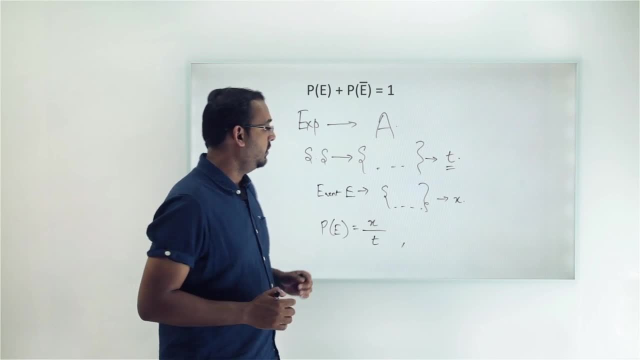 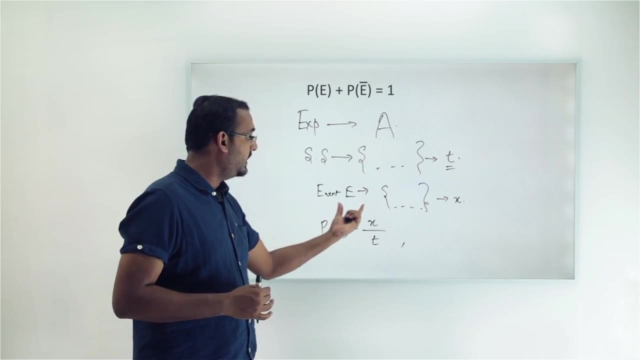 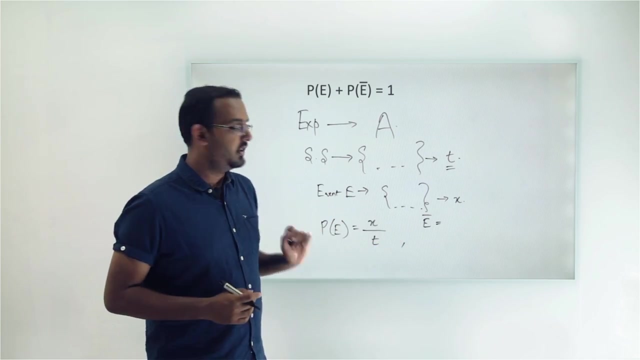 E are x. So now can you think of the probability of this event E not happening. So now can you think about it, what are the cases which will be favorable to the event E not happening? So, if you think about it, the cases which are unfavorable to the event E are going. 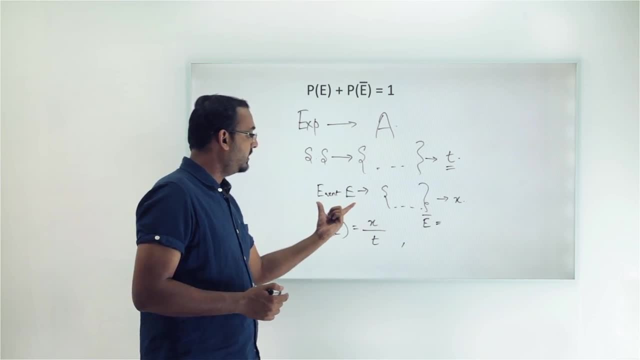 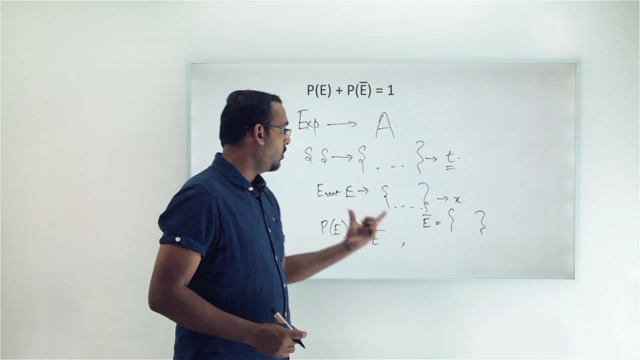 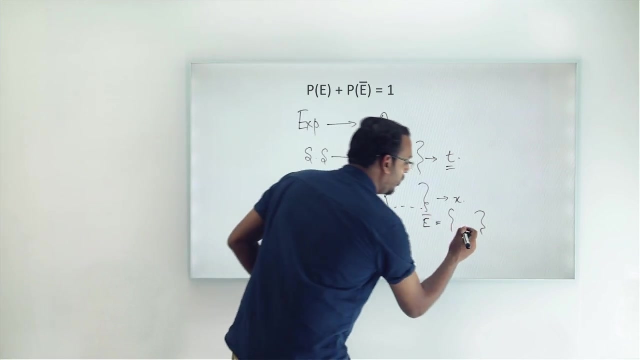 to be the cases which will be favorable to the event of E not happening. So this set will contain all the values of the sample set which are not present in the event E subset. So all the values that are present here. they will be a total of T minus X. 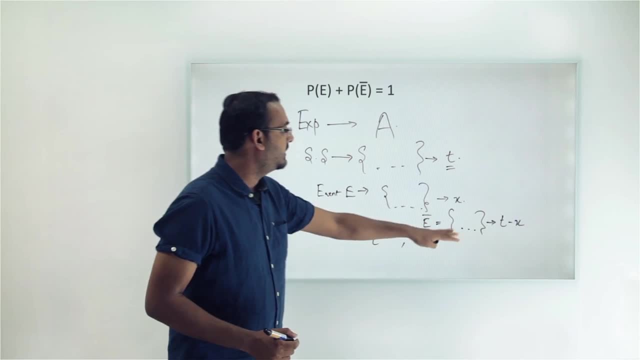 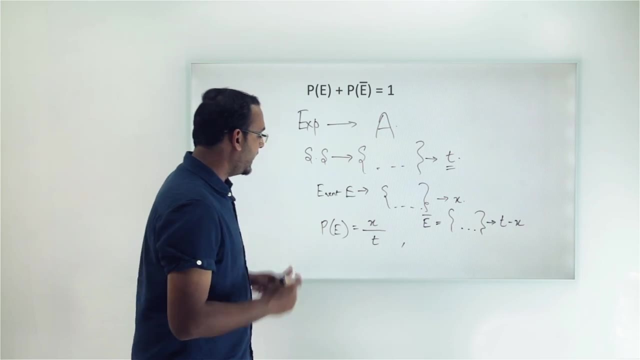 Why? Because X cases are favorable to E and there are a total of T cases. So the cases which are not favorable to E are going to be T minus X. So now, if we calculate the probability of E not happening, we can see that this value is going to be equal to T minus X.